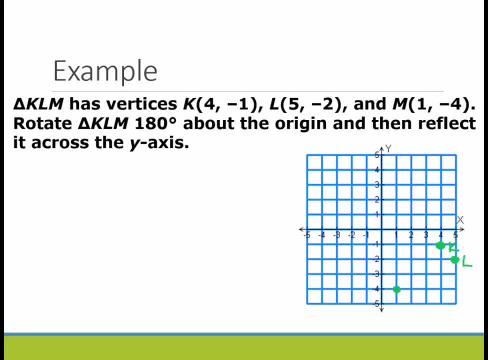 And then 1, negative 4.. So here's our triangle, And the first thing we're going to do is rotate 180 degrees. Now, if you remember your rules, remember to rotate something: 180 degrees. all you've got to do is change the signs on your X's and Y's. 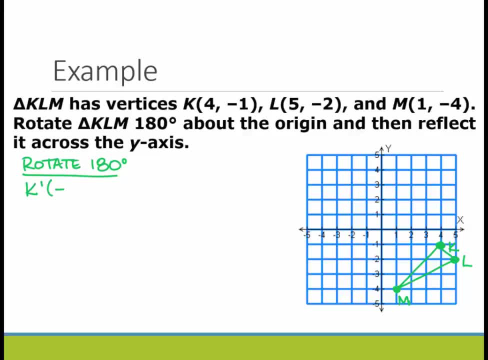 So K prime is going to be negative, 4, positive, 1.. L prime is going to be negative, 5, positive, 2.. And M prime is going to be negative, 1, positive, 4.. So if we put these on here, 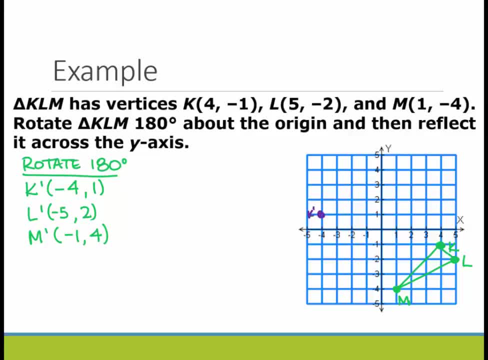 Negative 4, positive 1.. Negative 5, positive 2. And negative 1, 4.. So that's the rotated one, And now we want to flip this across the Y axis. So remember, when something flips across the Y axis. 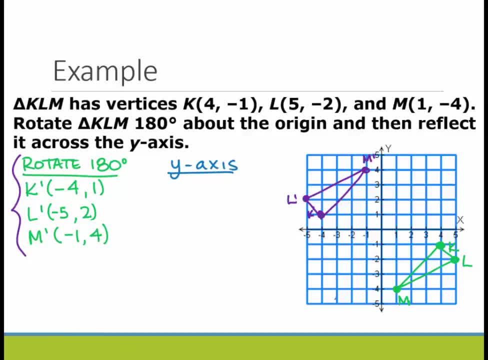 you keep the Y values the same, but you change the X values. So K double prime is going to be: keep the Y values the same, so that's a 1, but you make that a positive 4.. So change the sign on the X's, keep the Y's the same. 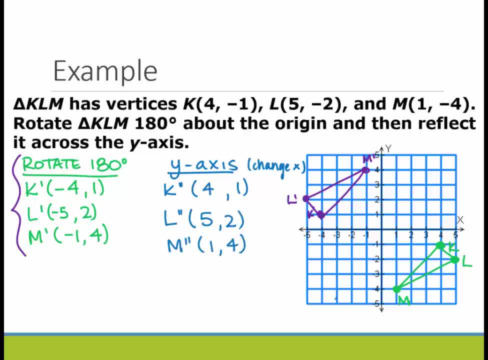 Change the sign on the X's, keep the Y's the same And we should imagine that our shape is going to be somewhere over here in quadrant 1.. So K is at positive 4, 1.. L is at 5, 2.. 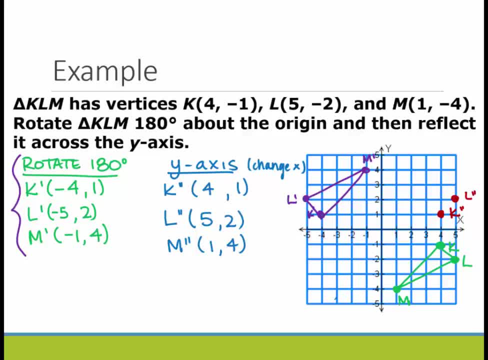 And M is at 4, or 1, 4.. So when we connect these, this red shape right here is our image, That's our answers, everything that's over there. So basically, we just did two things to it all in one problem. 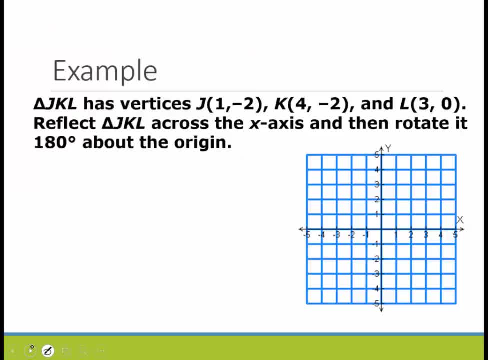 So let's do a different one: JKL. so same letters. reflect it across the X axis first and then rotate it 180 degrees about the origin. Now you will get different answers depending on the order that you do this, So make sure you do it in the correct order. 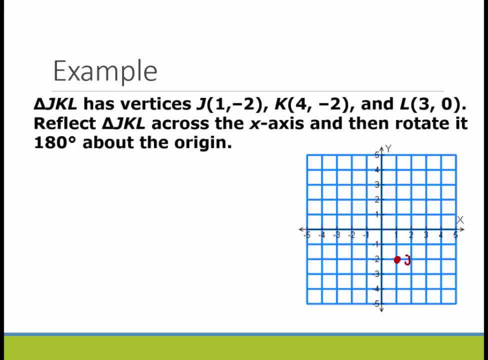 So over 1 down 2 is J, Over 4 down 2 is K And L is 3, 0.. Here's my original shape. First thing I want to do to it is reflect it across the X axis. So remember, if we do something across the X axis, you change your Y's. 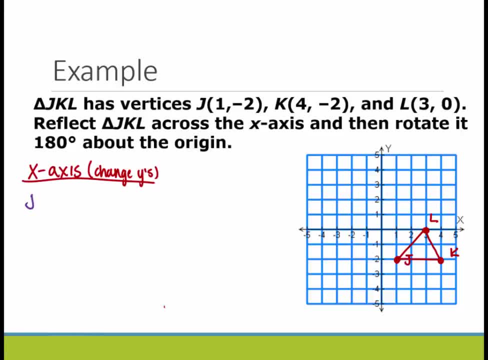 So our new points, Our new points are going to be: keep the X's the same, make the Y's positive. Okay, Should be: X is the same, Y is positive, L X is the same, Y is positive, So that 0 doesn't move. 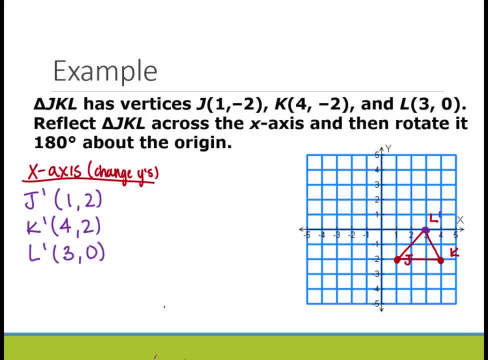 Because it's on the X axis. this is also L prime. So then, J- I'm going to go over 1, up 2.. K- I'm going to go over 4, up 2.. So here is my in between shape. 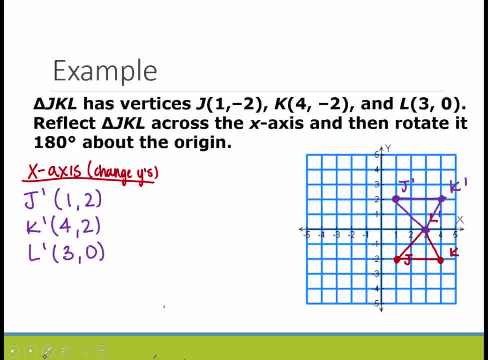 And then I'm going to rotate it 180 degrees about the origin. So remember, 180 degrees means that you make your X's and Y's both negative, So this will be negative 1, negative 2.. K will be at negative 4, negative 2.. 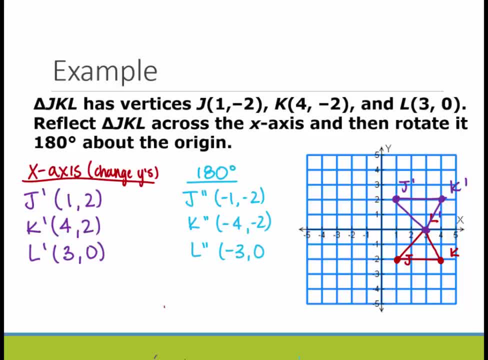 And L will be at negative 3 and 0.. You can't make negative, So it's just at 0.. So negative 1, negative 2.. K is negative 4, negative 2.. And L is negative 3, 0.. 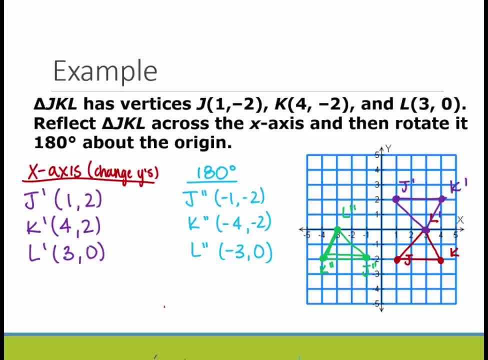 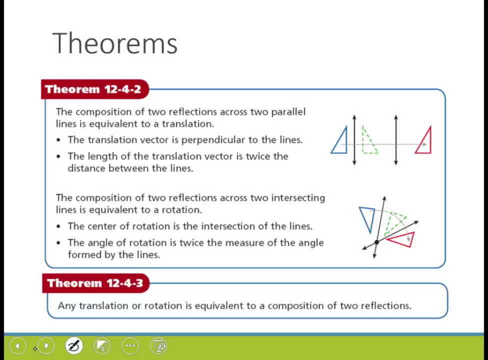 So this right here is our final shape. So here's some theorems. The composition of two reflections across two parallel lines is equivalent to a translation. So think about that for a second. If you flip something over and then flip it over again, you get the original image. 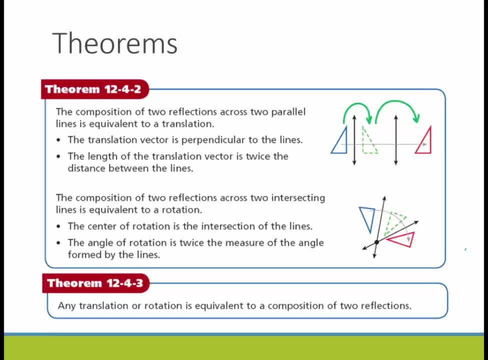 So this got flipped over and then flipped over again. So this triangle is exactly the same as this one, And now it's just a translation. The key thing is these two lines have to be parallel. in order for that to happen, The translation vector is perpendicular to the two lines. 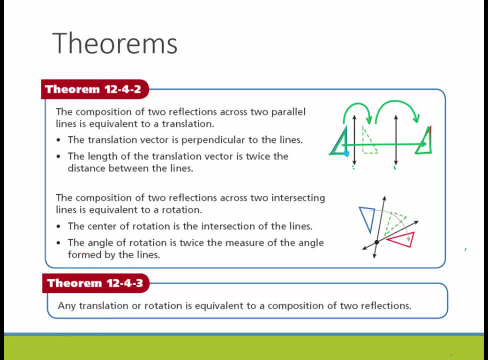 So the translation vector is, if I go from this point to this point, same point, but on image and preimage it's perpendicular to those two parallel lines, And then the length of that is twice the distance between the lines. So whatever this distance is, here this whole distance is twice as big. 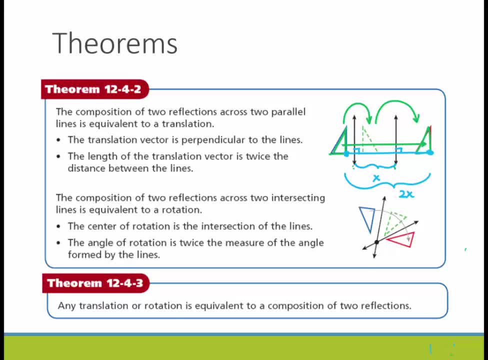 The composition of two reflections across two intersecting lines is equivalent to a rotation. So I flipped it over this one and then flipped it over another one, And because these two lines cross, it's really just like I rotated this original image. The center of rotation is the intersection of those lines. 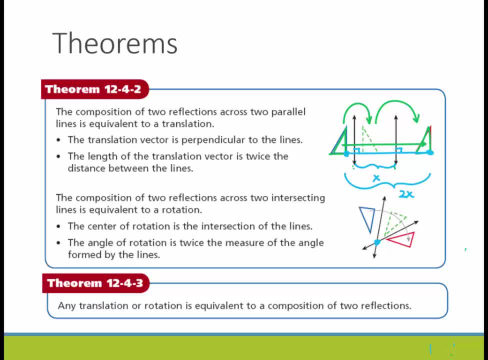 So is where we usually like it to be. And the angle of rotation is twice the angle measure of the angle formed by the two lines. So, whatever this angle is this: that it rotated is twice the angle measure of the two lines. double that, And then you need to remember that any translation or rotation is equivalent. 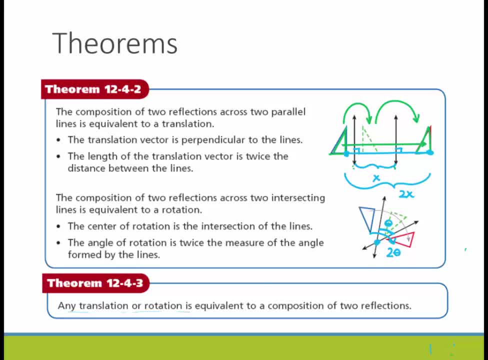 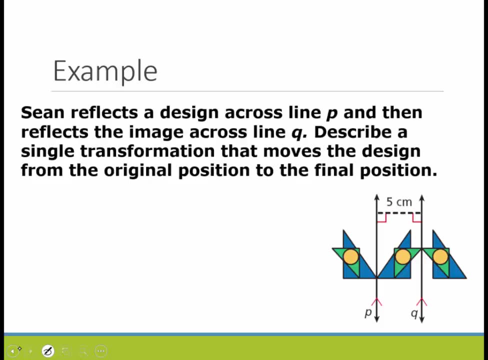 to a composition of two reflections. That's basically what this is saying. Two reflections equal a rotation, two reflections equal a translation. So let's say, Sean reflects a design across line P and then reflects it across line Q. So two reflections Describe. 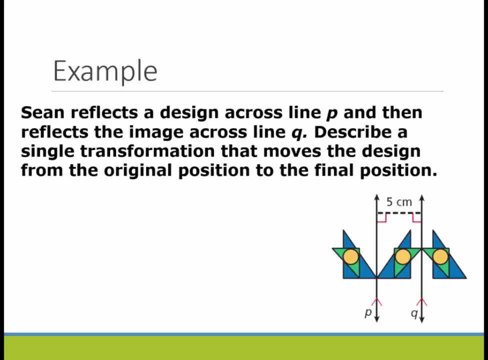 a single transformation that moves the design from the original position to the final position. So here to here, here to here and here to here. So, because he reflected it twice, two reflections equals a translation And if I want to describe this, they told me the distance. 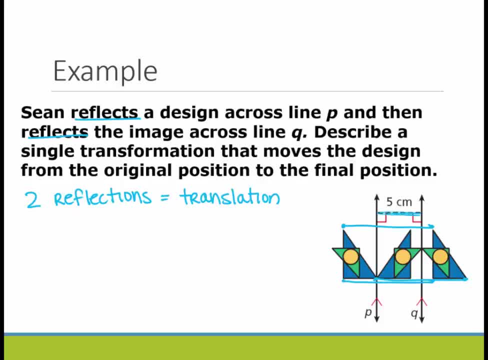 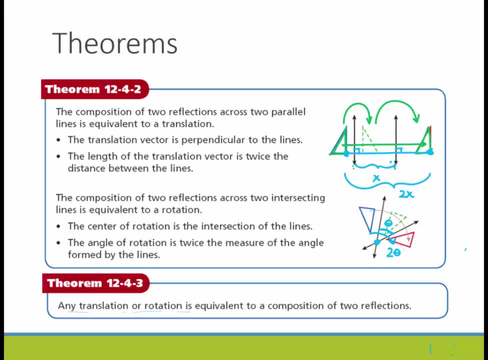 between these two parallel lines is five centimeters, This translation has to be double that. So translation of ten centimeters is what will get us to that final position. And remember, that just comes from this theorem that whatever this distance is between these two parallel lines double. that is the distance, the entire.